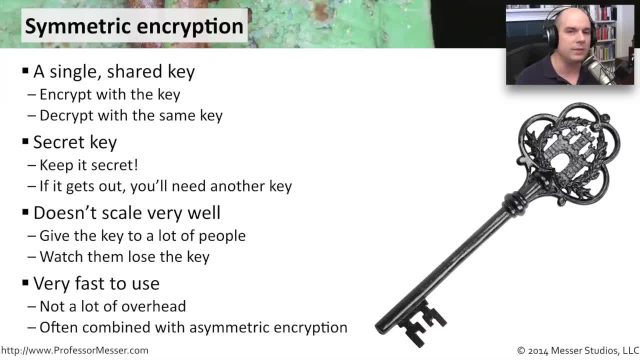 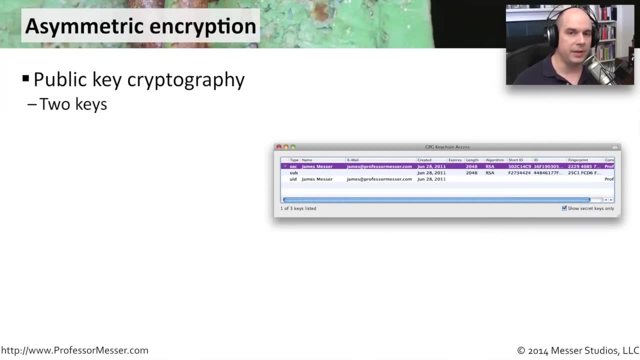 see these combined. You'll see asymmetric encryption combined with symmetric encryption to be able to have not only a secure environment where data is protected, but also have one that works very, very quickly and very, very efficiently. The other type of encryption that you'll commonly see is asymmetric encryption. You'll also hear this referred to. 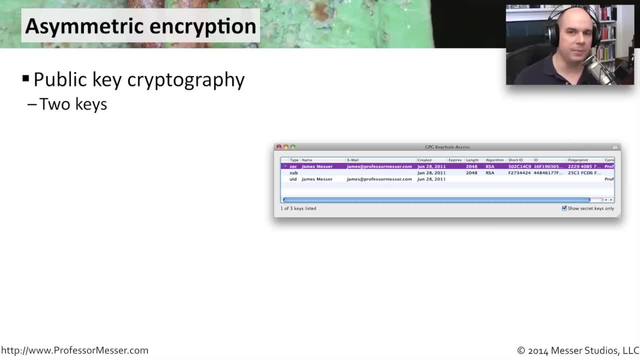 as public key cryptography, And you'll understand why in just a moment. This type of encryption method has really only been around since the 1970s, So in the world of encryption it's a relatively new capability And it has allowed us to do quite a number of things. 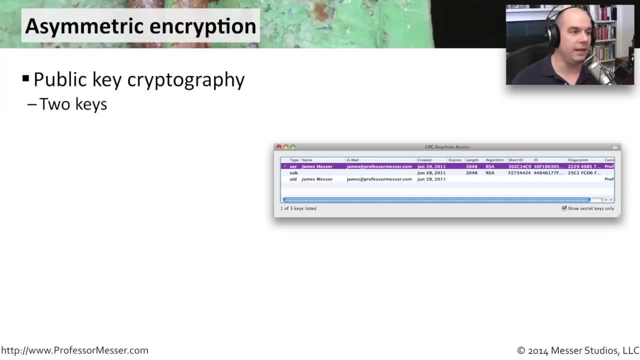 in our technologies, There are two keys needed. in asymmetric encryption, If you recall, in symmetric encryption you had exactly the same key, But in asymmetric encryption, as the name implies, you have two keys. You have a private key And this private key is something. 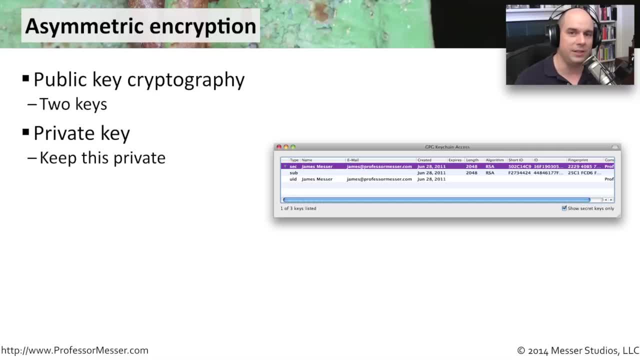 as also this name implies, you want to keep private. Nobody gets their hands on the private key except for you. You would not share this private key with someone else. You would not give it to someone else. Nobody else needs this private key, The key that. 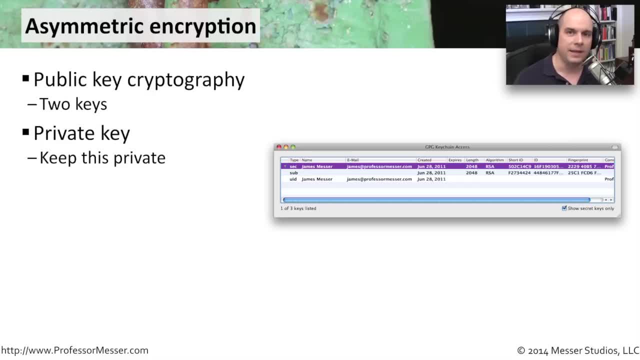 you're going to give to everyone else is one called a public key. Give it to everybody, Put it on a public server, Post it on your website, Stick it on your Facebook page. Everybody should have access to this public key- Nobody, but you should have access to the private key. 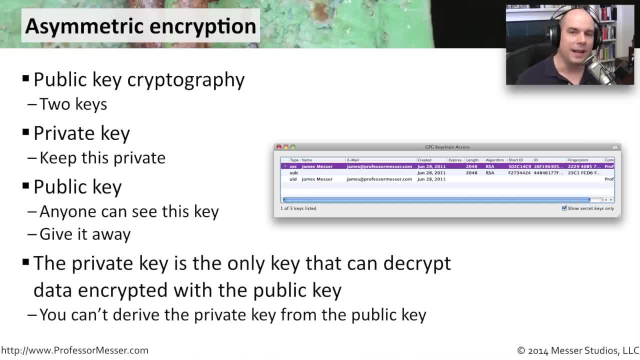 And that's because the public key is one that allows people to send you information in an encrypted form, But the private key is the only key that can decrypt that data, And that makes this a very interesting method of storing and encrypting information. Because if 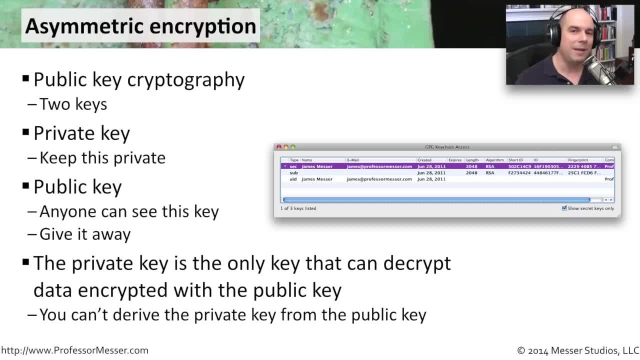 somebody was to encrypt data with your public key, they would not be able to decrypt it. Nobody would be able to decrypt it, even if somebody got their hands on it somewhere along the way. The only way to decrypt it is with that private key, And that's why it is so important to keep that key private. 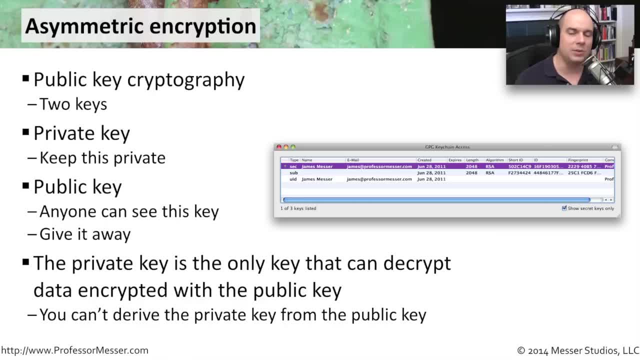 Not only is it private, we usually will put a passphrase associated with it. We make sure that that key is very, very secure and nobody gets their hands on it, And in that way you can be relatively public with the information that you're sending. You don't have to worry about it so much.